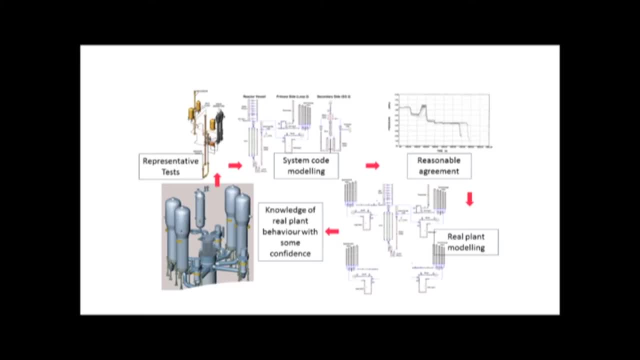 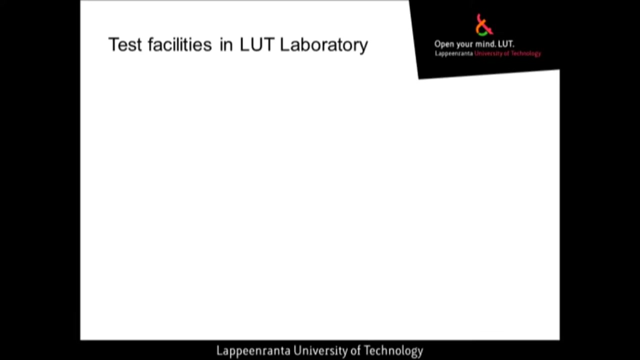 recently, Fukushima. The results of thermal hydraulic experiments are used for validation of the computer codes that model the behaviour of nuclear power plants. Validation ensures that real plant calculations can be performed to acceptable accuracy. When it was constructed, the main objective of the REWET experiment was to observe the 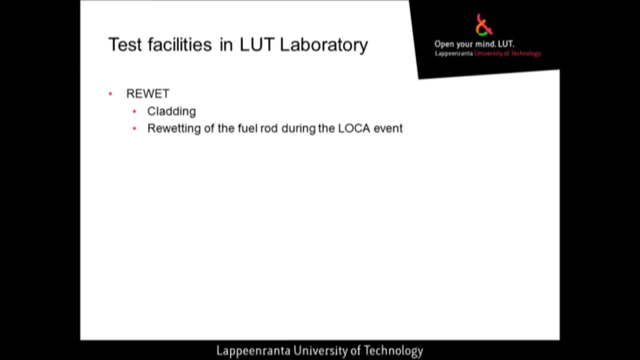 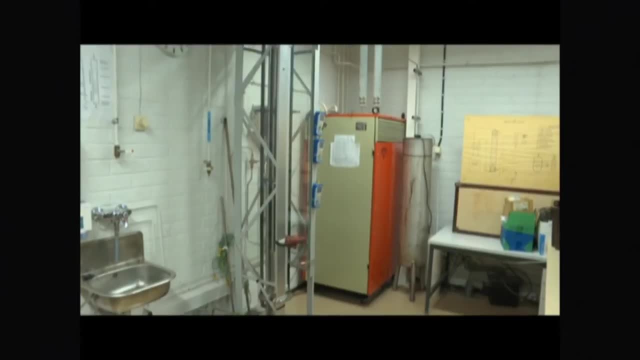 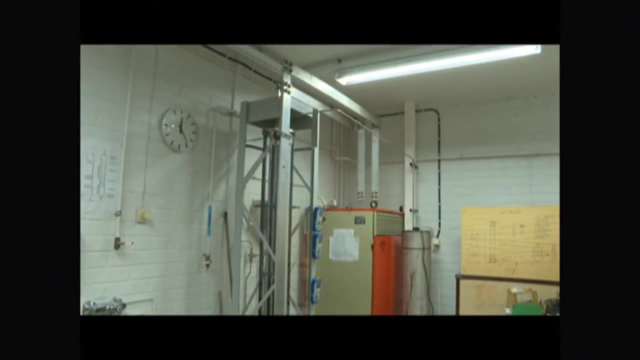 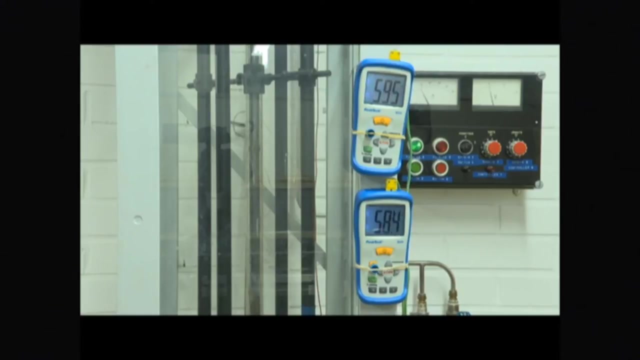 test facility was to investigate the fuel rod re-wetting process and derive heat transfer coefficient values for heat transfer from the rod surface to the coolant. The effect of nitrogen dissolved in the coolant was also studied. The facility is now used only for demonstrations and student work. The re-wet test facility. 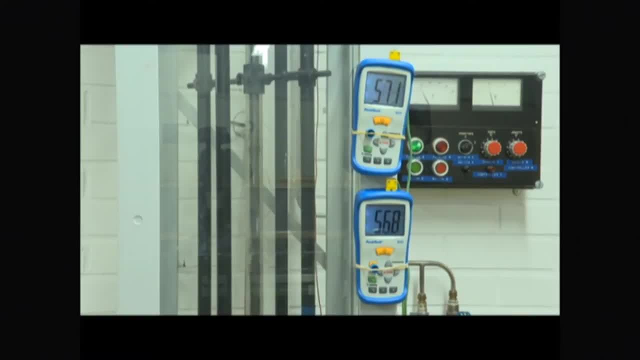 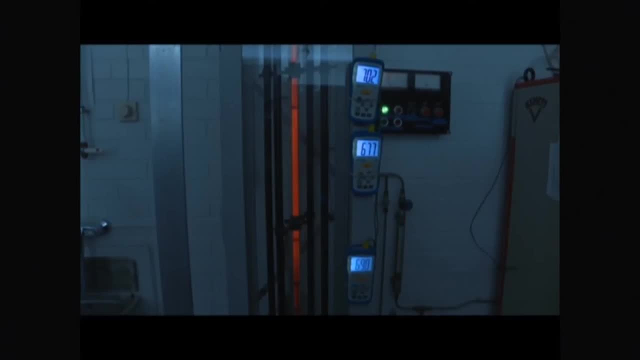 has three rods in the core with a total heated length of 1.5 meters. The transparent tube surrounding the rods allows the re-wetting phenomenon to be easily observed. The maximum heating power of one rod is 2000 watt and the initial cladding temperature. 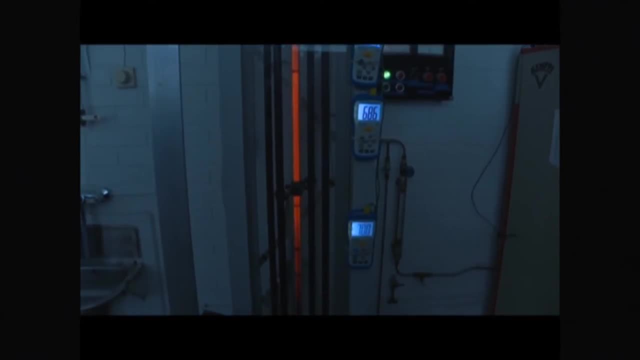 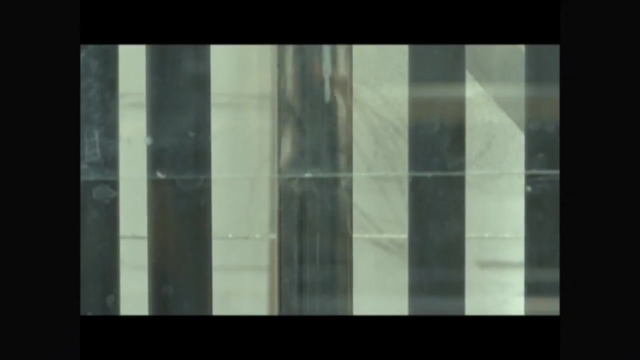 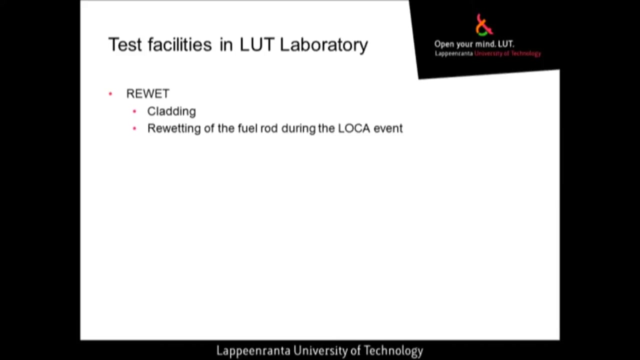 at the beginning of re-flood is between 300 and 900 degrees Celsius. The temperature of the injected coolant can be varied from 20 to 80 degrees Celsius. The PWR PacTel test facility has been designed and constructed to model the thermal hydraulics of an EPR type. 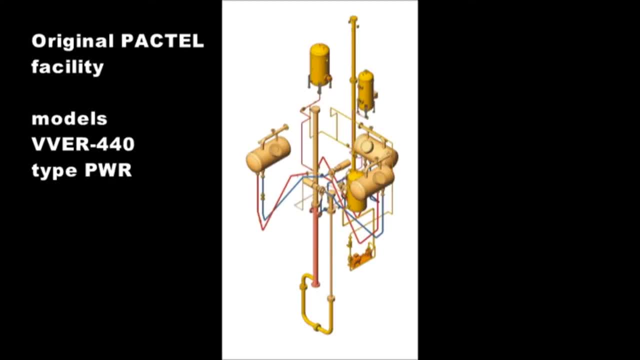 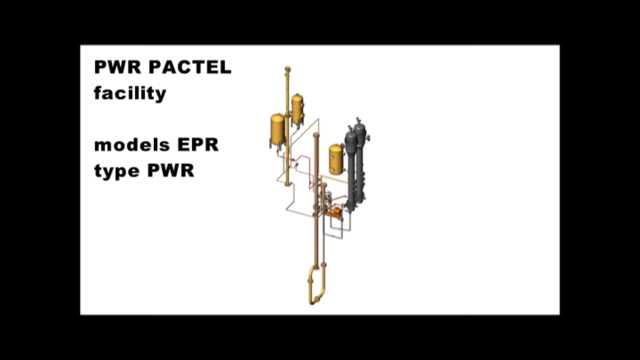 pressurized water reactor. A significant aspect of the design of the facility is the use of some parts from the original PacTel facility, which is used to simulate the behavior of the Soviet designed VVER 440 pressurized water reactors currently in use in Lovisa, Finland, The PWR PacTel test facility. 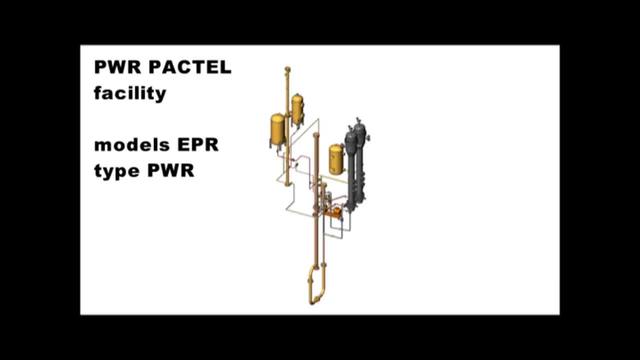 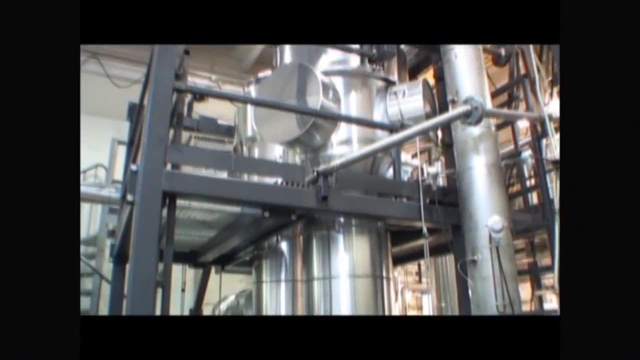 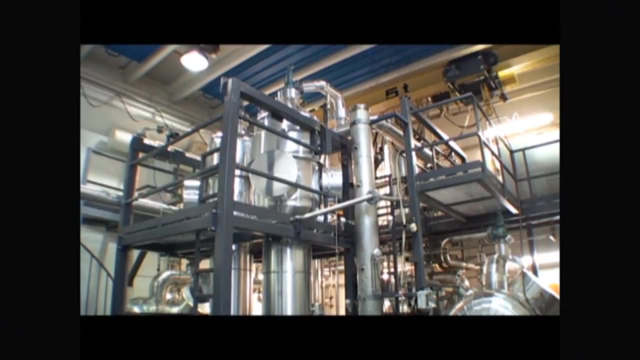 comprises a reactor pressure vessel model, two primary circuit loops with vertical steam generators, a pressurizer and emergency core cooling systems. PWR PacTel experiments aim in particular to gain experience of the thermal hydraulic behavior of the EPR primary circuit, especially the steam generators. 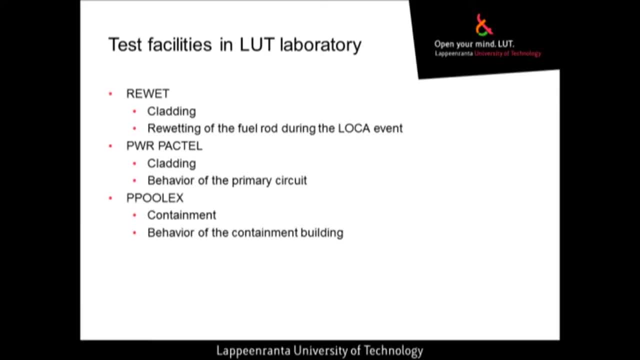 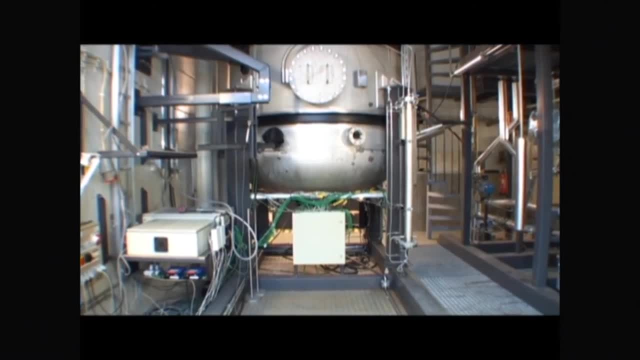 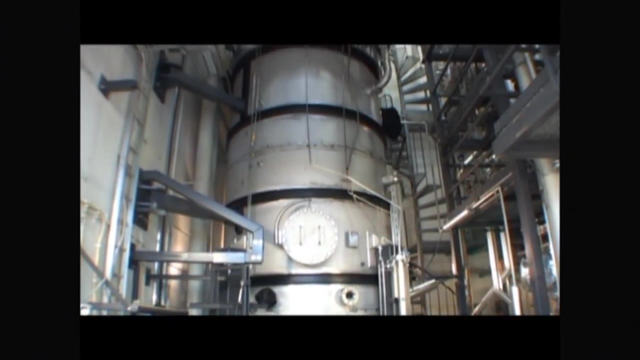 The P-Poolex test facility models a boiling water reactors containment system and is used for condensation studies. The main component of the test facility is the approximately 7.5 meter high cylindrical test vessel. The facility has dry well and wet well compartments. 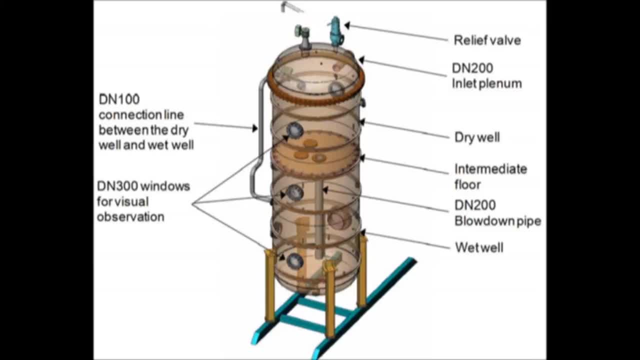 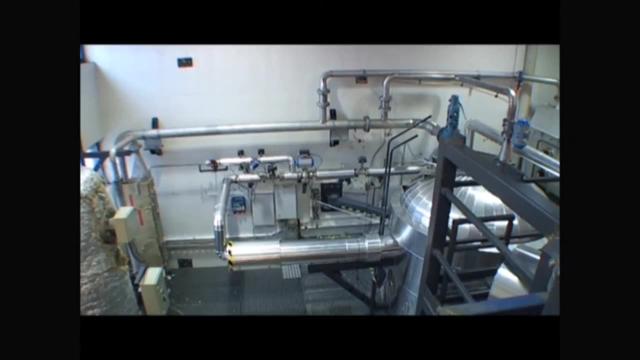 separated by an intermediate floor. Gas is directed from the dry well to the wet well by a vertical blow down pipe attached underneath the floor. The vessel sections modeling the dry well and wet well are volumetrically scaled based on the containment systems of the two. 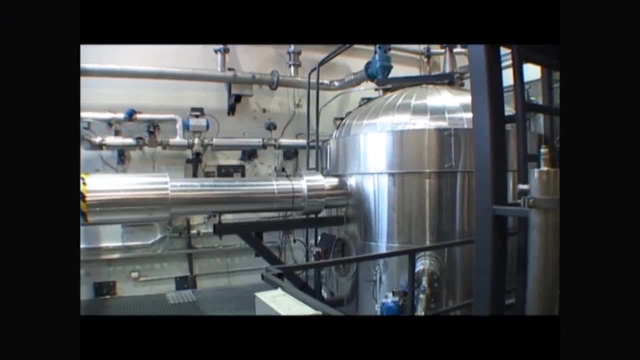 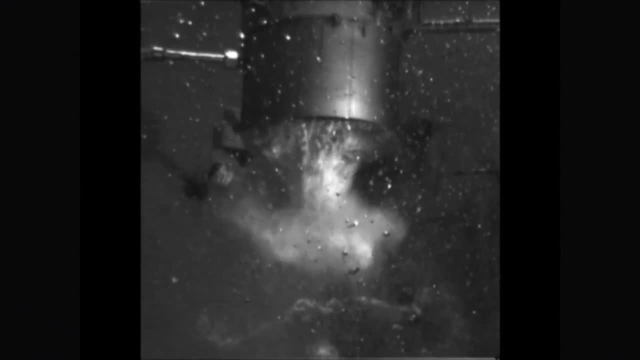 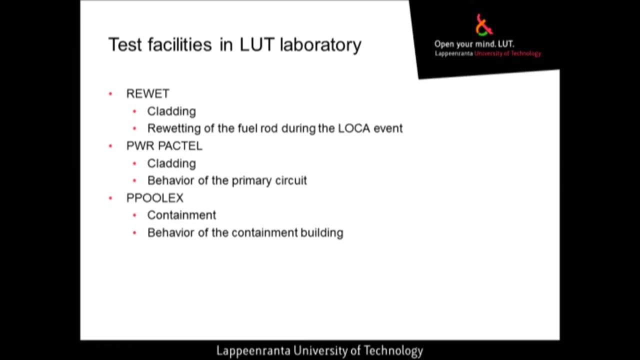 boiling water reactors at the Olkiluoto plant in Finland. The test facility is able to withstand the considerable structural loads caused by rapid condensation of steam. The HYPE test facility is designed to study two-phase flows in an inclined pipe and to support experimental research on advanced measurement techniques. 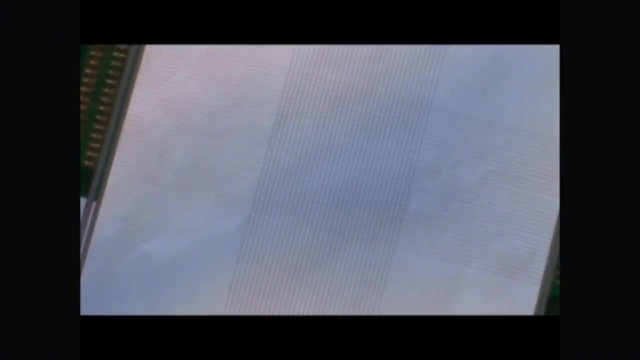 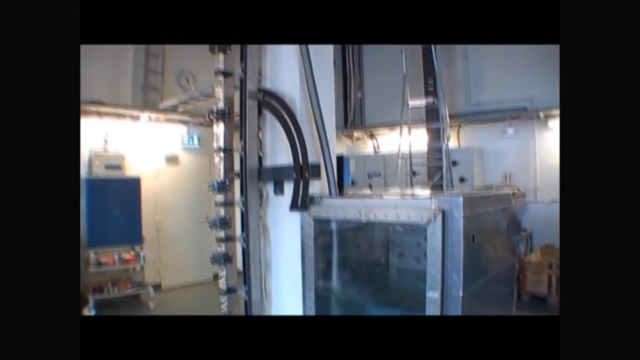 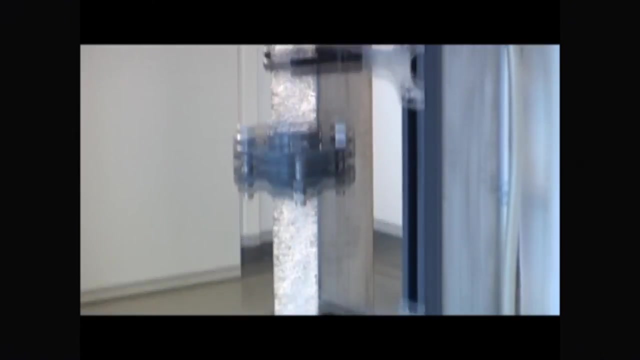 such as particle image velocimetry and the use of wire mesh sensors. The test facility consists of a transparent pipe section, a water storage tank and piping. The pipe section is made of acrylic pipe with an inside diameter of 50 mm and the alignment